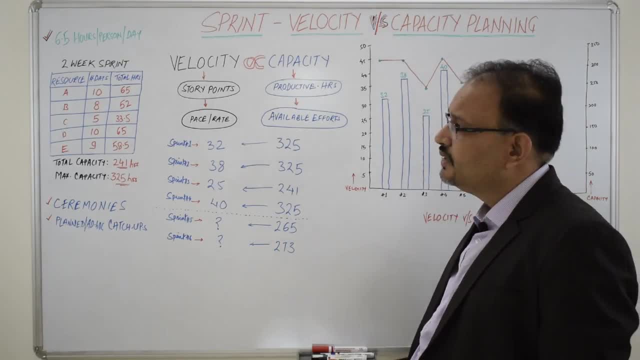 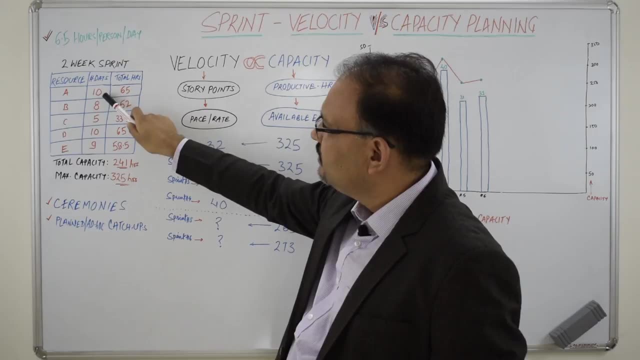 Let's see one example. How do we do the capacity planning? Let's assume there is a 2 weeks sprint, that is 10 days. There are 5 resources: A, B, C, D, E. Resource A is available for full 10 days, So his productive available hours are 10 multiplied by 6.5. 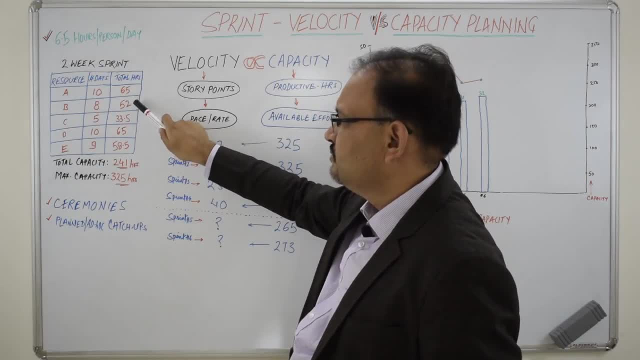 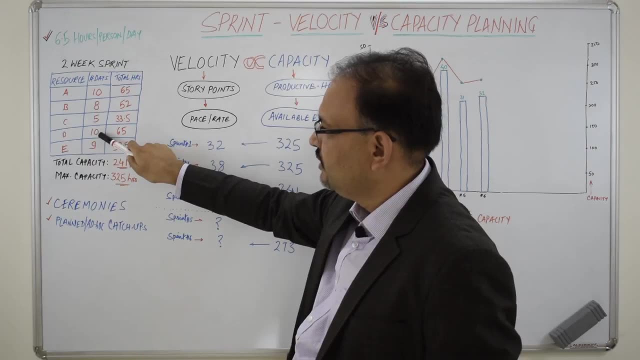 B is absent for 2 days, So his available productive hours are 52. He is available only for 5 days, that is 33.5.. He is again available for full 10 days, so that is 65.. He is absent for 1 day, so 58.5.. 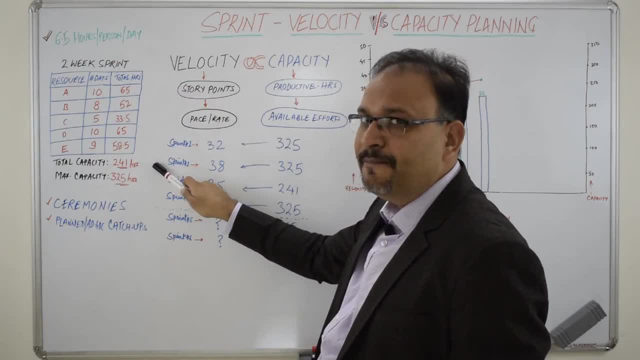 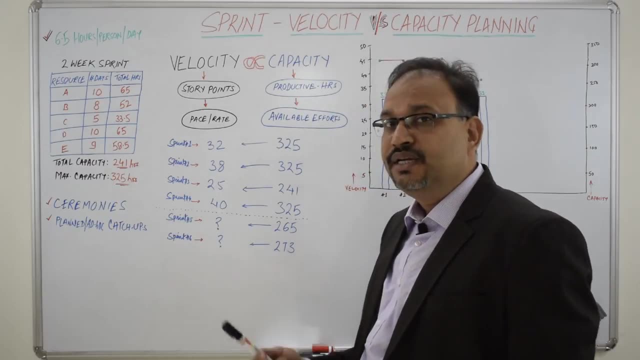 The total of these hours becomes the total capacity of the team for that sprint. What is the maximum capacity of the team? If everybody would have been present in the office for full 10 days, everybody would have clocked 65 hours for the productive team. 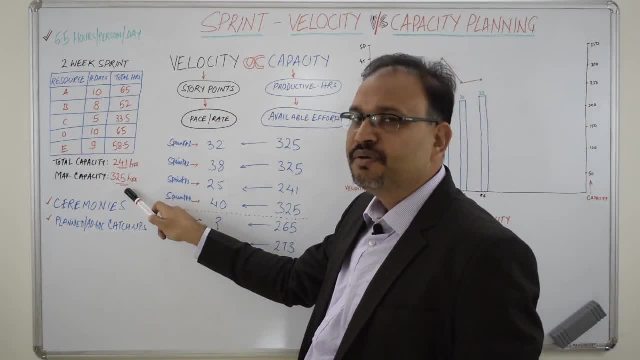 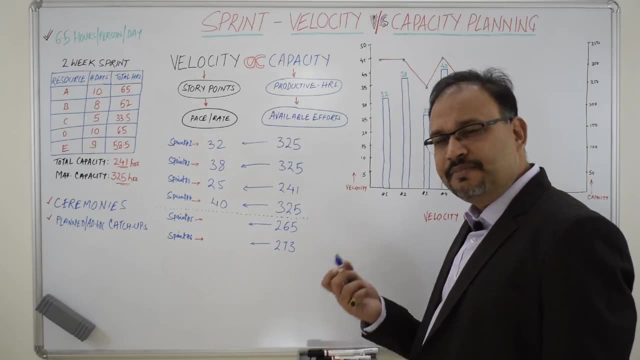 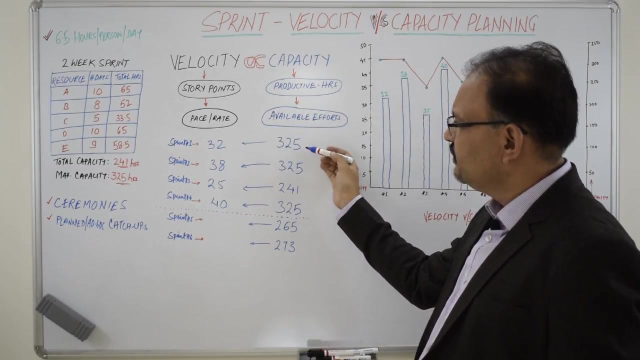 The sum of that would have been the maximum capacity of the team, that is, 325.. Now let's see how does the relationship between velocity and the capacity evolves? sprint over sprint. In the very first sprint team is available in full capacity, that is 325, and they are knocking off the velocity of 32. story point: 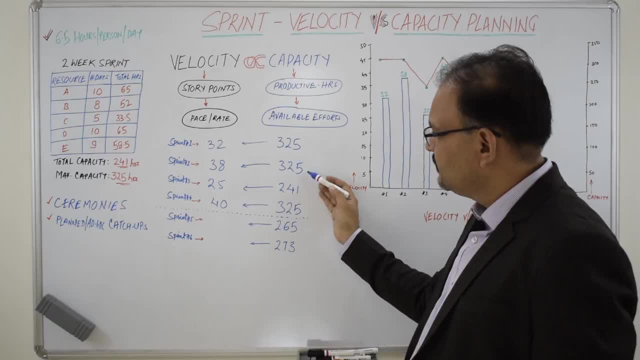 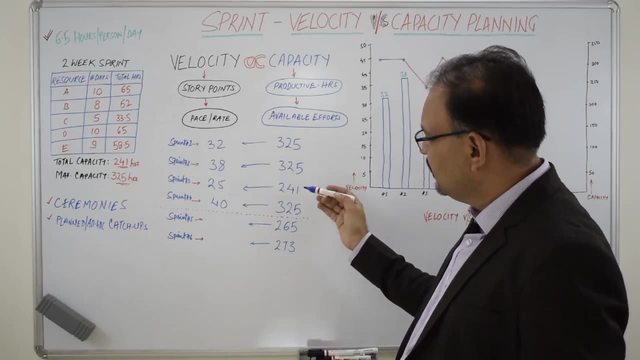 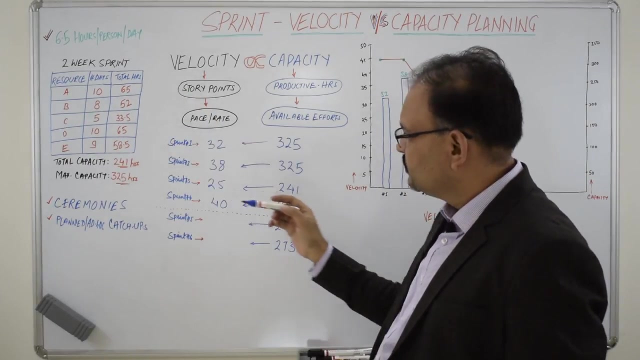 In the second sprint again, team is in full capacity and they are knocking off the velocity of 38 story point, which is a slight improvement there. In the third sprint, team is only available for 241 hours as some of the members has gone on the leave, so they are knocking off a velocity of 25 story point. 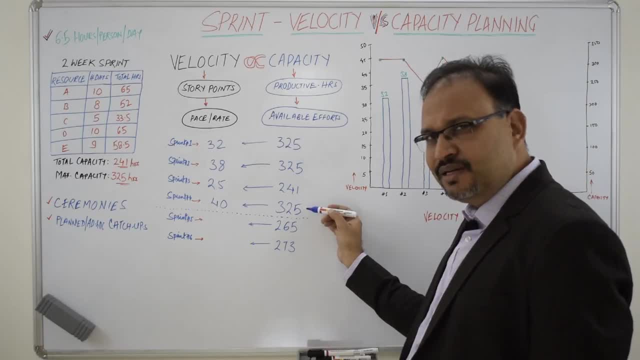 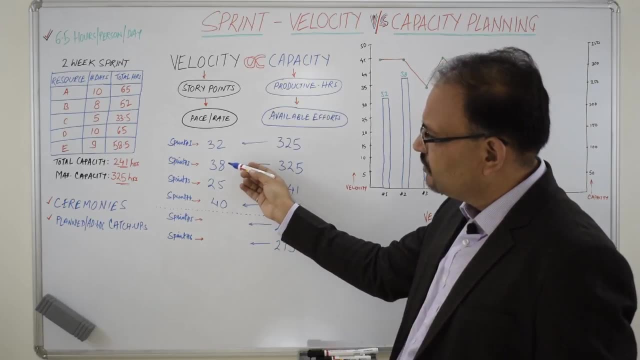 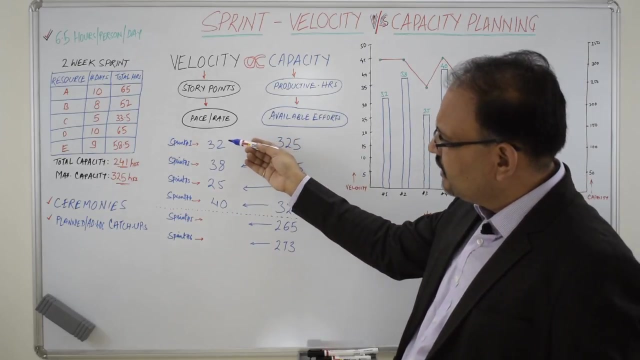 In the fourth sprint again, team is in full capacity, everybody is present for 10 days. they are knocking off a velocity of 40- story point- which is a slight improvement from 38.. Now we can see a trend emerging here: When the team is in full capacity, they are knocking off a velocity of 32, and then 38 and 40. 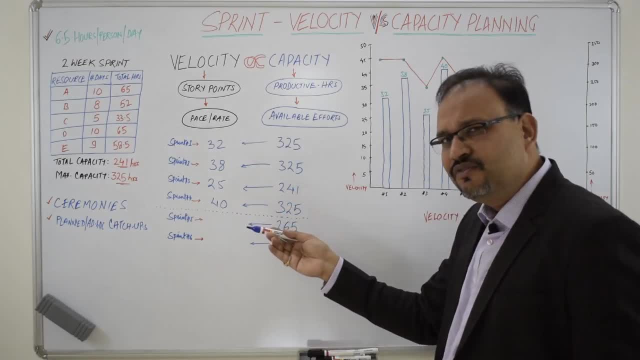 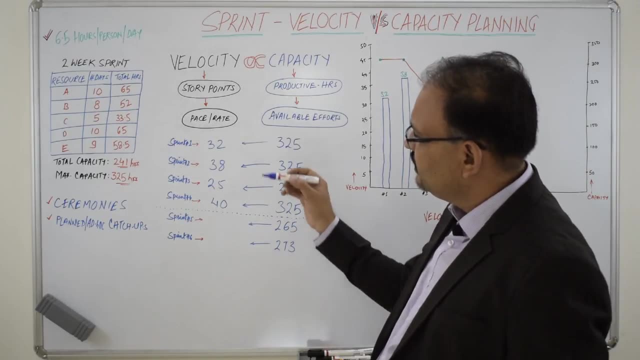 What we can do. We can take the average out of this velocity and figure out the velocity of the team there. Or, to be more realistic, what we can do is we can ignore the lower end side of it and the higher end side of it. 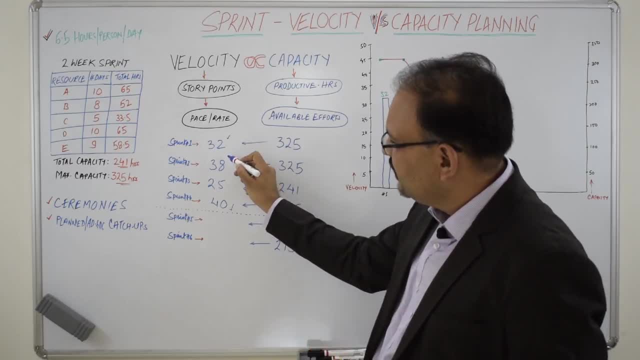 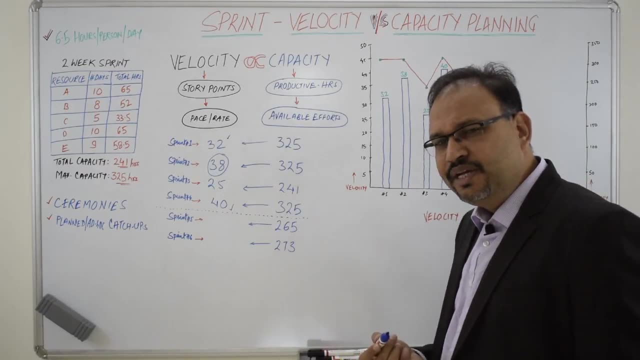 and we can go with the middle figure of the velocity, that is, 38.. So 38 becomes the velocity of the team, based on which we can make predictions for the upcoming sprints, as long as we know the capacity of the team. 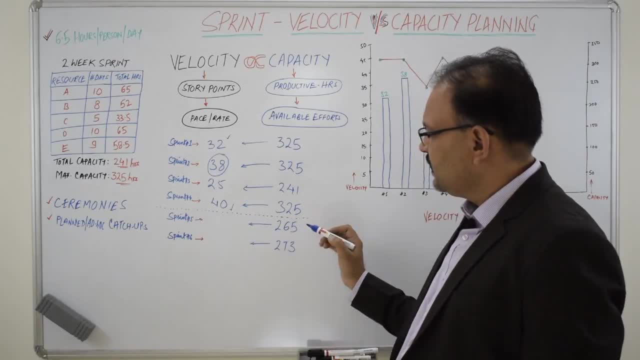 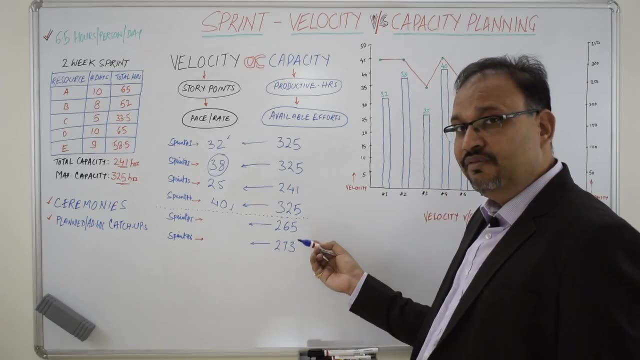 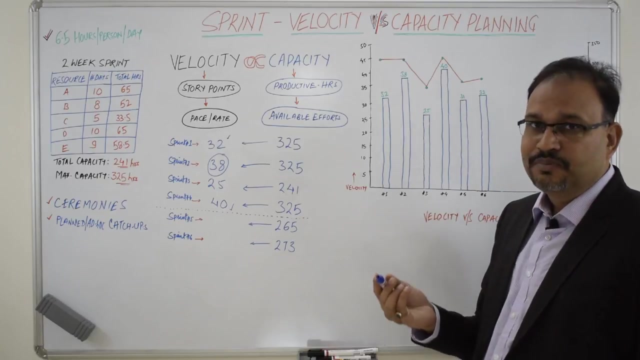 For example, for sprint 5, we know the capacity is 265.. For sprint 6, we know the capacity is 273.. We can easily calculate the velocity of the team and keep the client apprised on it, so that there are no surprises. 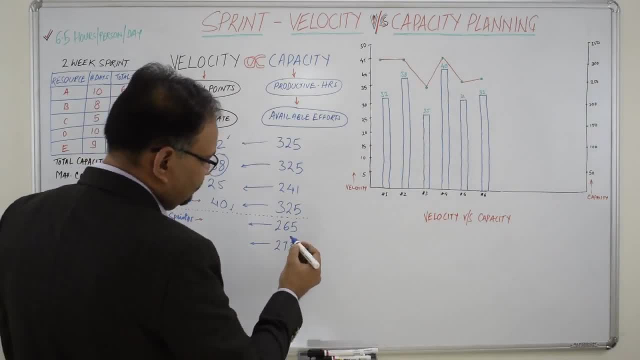 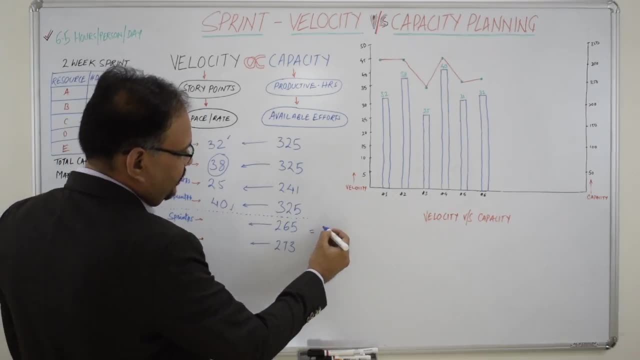 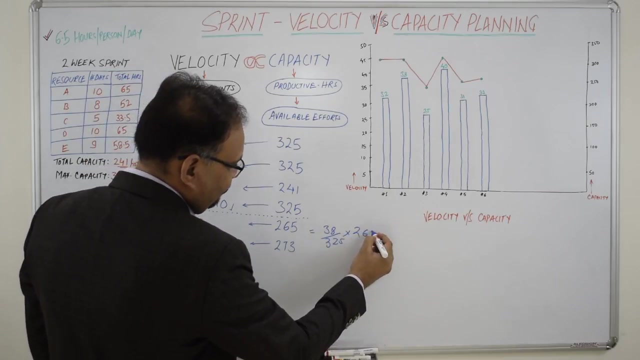 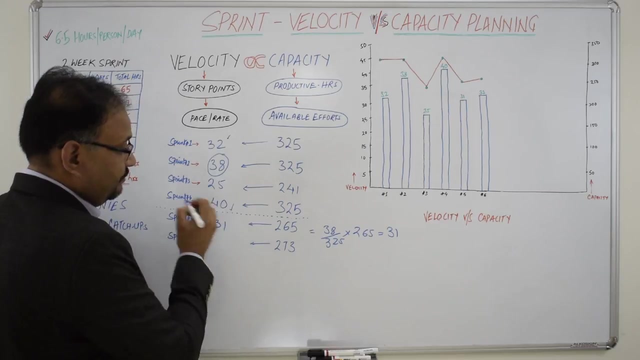 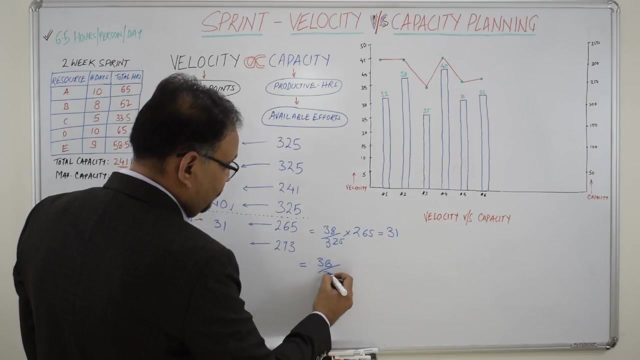 Let's see: When the capacity is 265, the velocity will be 38 divided by 325.. That comes out to be 31.. So 31 is the projected velocity for sprint 5.. For sprint 6, 38 divided by 325, multiplied by 273. 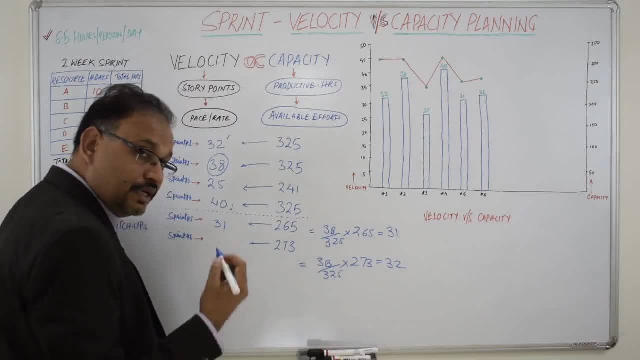 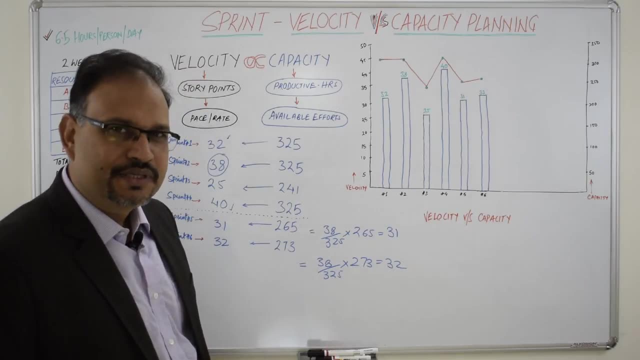 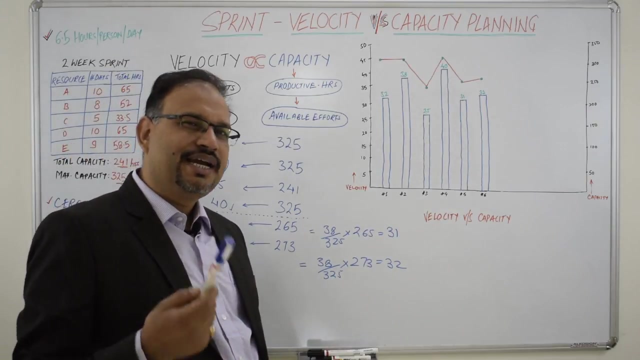 This comes out to be 32.. So 32 is the projected velocity of the sprint 6.. We can show the relationship between velocity and the capacity planning using this bi-directional chart. This chart will make more sense to the customer and they can set the right expectation from the team for the subsequent sprints. 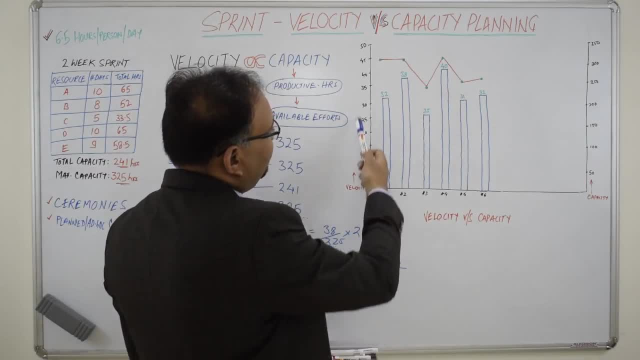 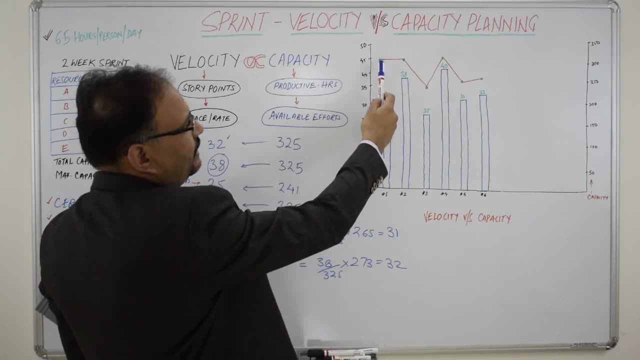 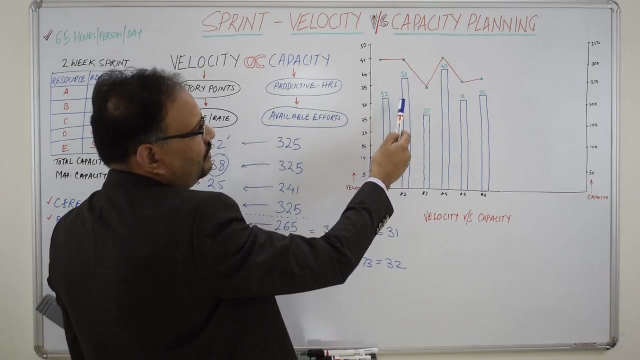 On the left-hand side is the velocity of the team. On the right-hand side is the capacity of the team. As you can see, for the first sprint the capacity is at 325 and velocity is just 32.. On the second sprint, velocity increased to 38, but the capacity remains the same, at the same level. 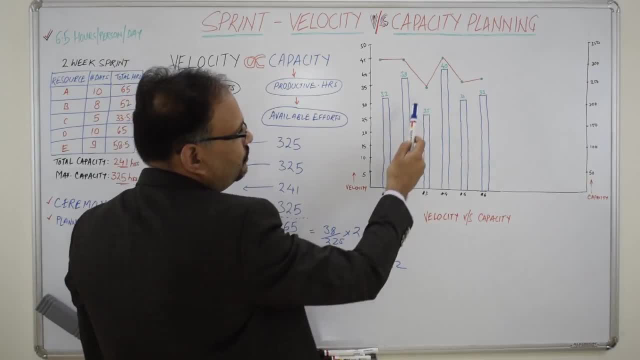 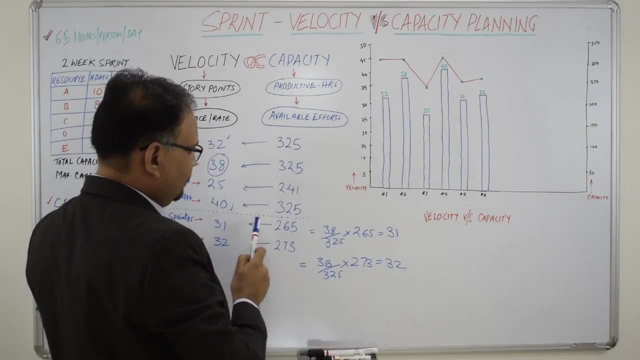 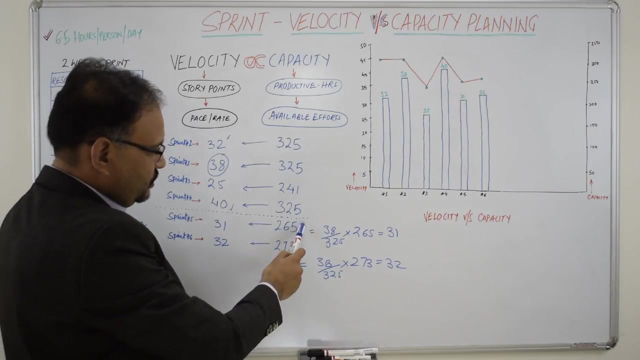 In the third sprint, the capacity is reduced down to 241 and velocity is also coming down to 225.. For the fourth sprint, the capacity has gone up to 325 and velocity also increased to 40.. Similarly, for sprint 5 and sprint 6, the capacity is 265 and 273.